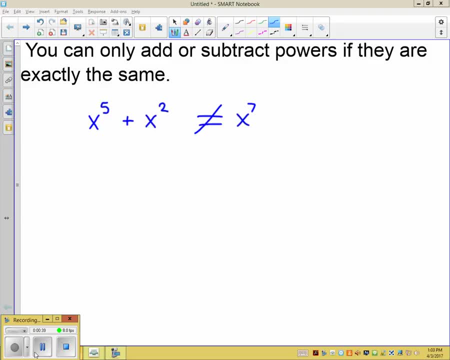 They're different powers. That means the base has to be the same and the exponent has to be the same. The base and exponent must be the same. So, for a different example, if I had x, If I had x to the power of 6 plus x to the power of 6, now they're the same power. 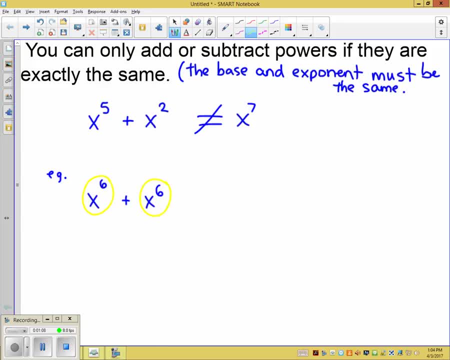 Because, remember this whole thing- the base with the exponent is a power. So since they're the same, I can simplify it further. So it becomes well, there's an imaginary 1 in front of this one and there's an imaginary 1 in front of that one. 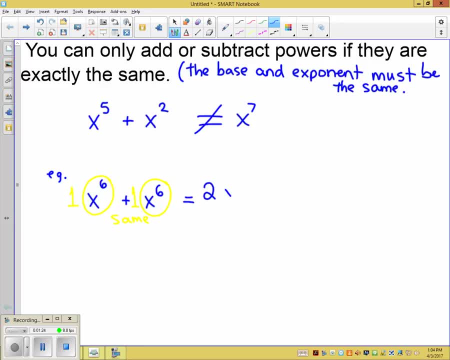 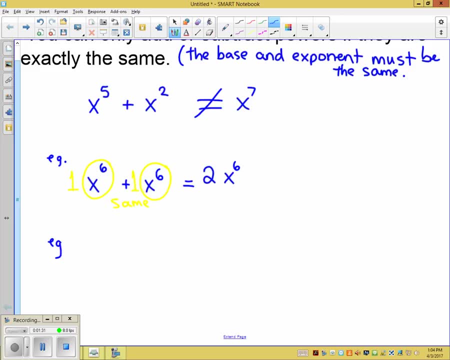 So 1 plus 1 is I've got 2 x's to the power of 6.. 2 x to the power of 6.. Example: what if I have 3b to the power of 2 minus 2b to the power of 2?? 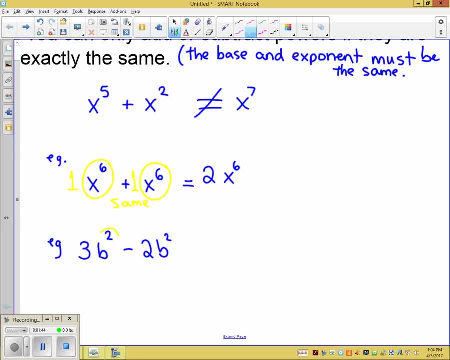 So the first thing you want to check is: are the powers the same? And yes they are. They're both b to the power of 2.. So then you look at the coefficients in front of them. I've got 3 minus 2 of those powers. 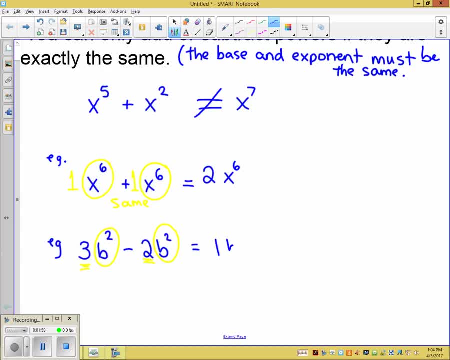 So that's 3 minus 2 is 1.. And then b squared, which can also just be written as b squared. We don't have to write the ones. Okay, so when it's adding or subtracting, the powers must be the same. 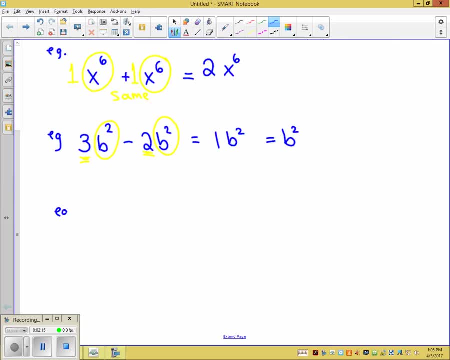 I'll do one more example with you. What if we have a fraction? What if we have 2 over 5 plus 2 over 5?? Let's change it up a little bit. Let's make this cubed and cubed on the left. 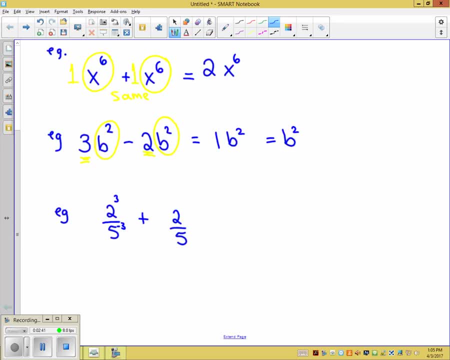 Right now the powers are not the same, Right, But if I put an exponent of 3 on this now, it'll be the same. It doesn't look like it yet, but when you apply that exponent into both parts, everything inside the brackets. 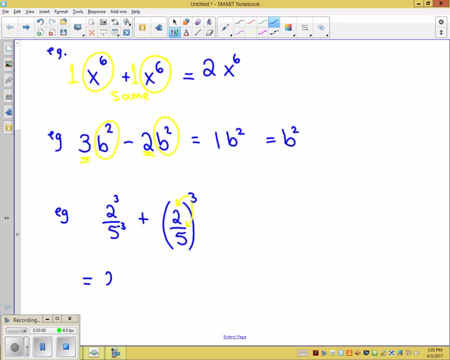 this becomes 2 to the power of 3 over 5 to the power of 3, plus 2 to the power of 3 over 5 to the power of 3.. So now these are equal. They're the same power. 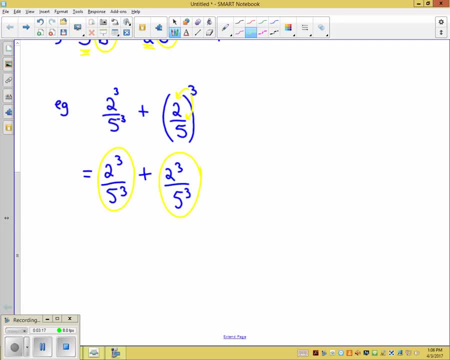 This and this are the same. They both have an imaginary 1 in front. So in total there's 2, of them 2, there's 2 to the power of 3 over 5 to the power of 3.. 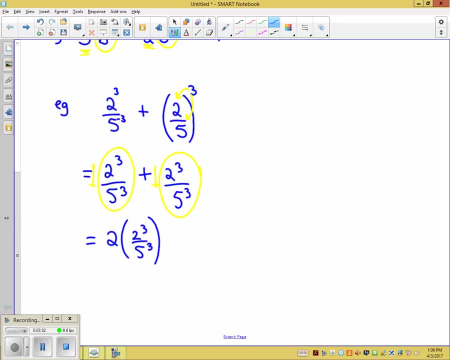 I put the brackets there just so you know. there's 2 of that power, So it's actually multiplying. When you What's the word I'm looking for? If you want to evaluate this, if you want to evaluate this, you can start by evaluating what's inside the brackets. 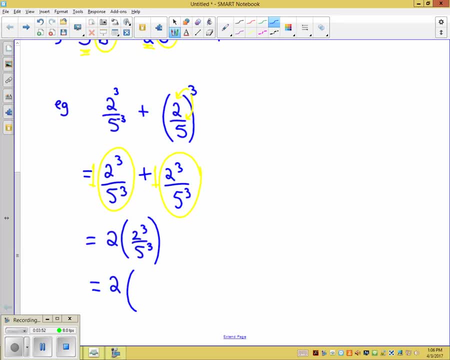 So 2 to the power of 3.. 2 times 2 is 4.. 4 times 2 is 8.. 5 to the power of 3 is 5 times 5 is 25.. Times 5 is 125.. 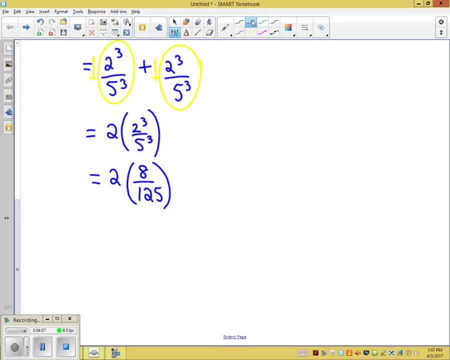 Then the rule here for multiplying is there's an imaginary 1 over any coefficient. So when you're multiplying you can multiply the tops, the numerators, and you can multiply the denominators. So this becomes 2 times 8 over. 1 times 25 is still 125. 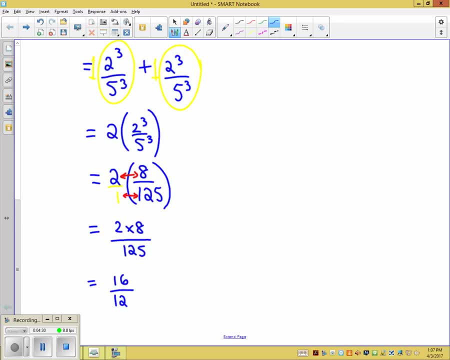 So this becomes 16. Over 125. And I can't simplify that any further. I don't think, because 125 ends in a 5, so it can only be divided by 5s, most likely, And 16 can be divided by 2.. 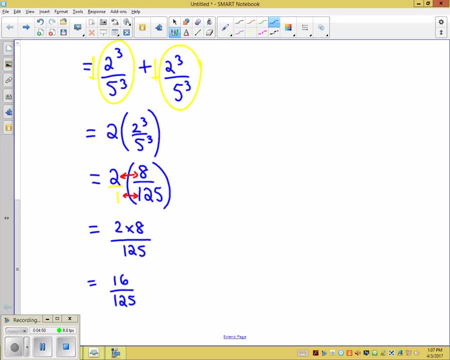 It can be divided by 4.. So I can check it out: 125 can't be divided by 2 or 4 without getting a remainder. So this is my final answer. This is evaluated Okay, And if I was asked to give my answer as a single, 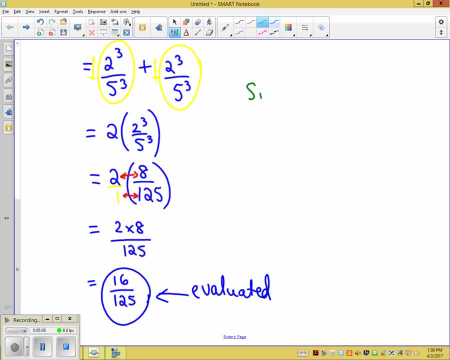 or simplify my answer as a single power. simplified as a single power, then the best answer for that would be: let's look back at what we had. This is close, So we're going to update it. It would be 2 and then 2 over 5.